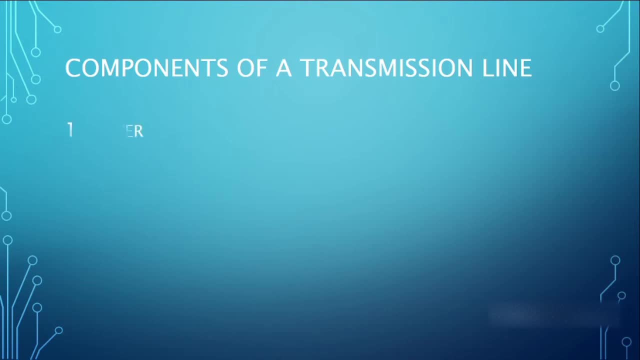 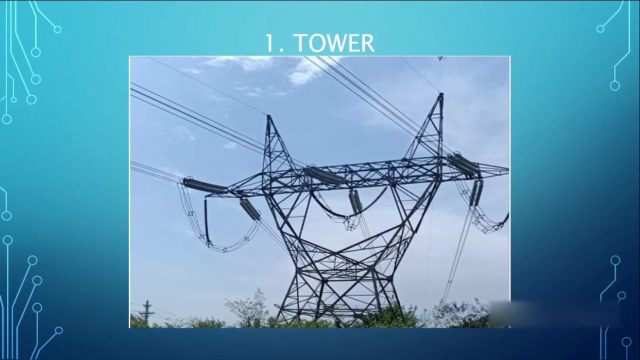 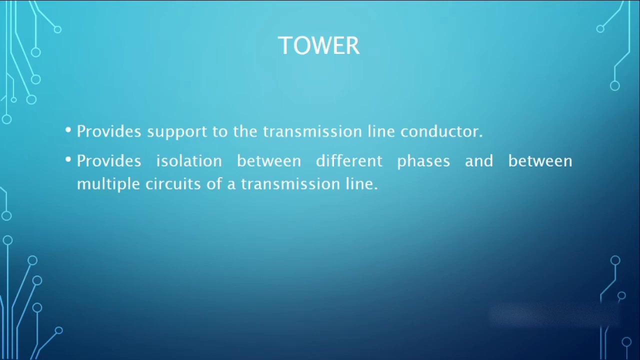 The main components of a transmission line are tower, conductor, earth wire or sky wire and allied hardware. First we explain. the tower Tower is the most important component of any transmission line. It is used to provide support to the transmission line and provide isolation between different phases and circuits of a transmission line. 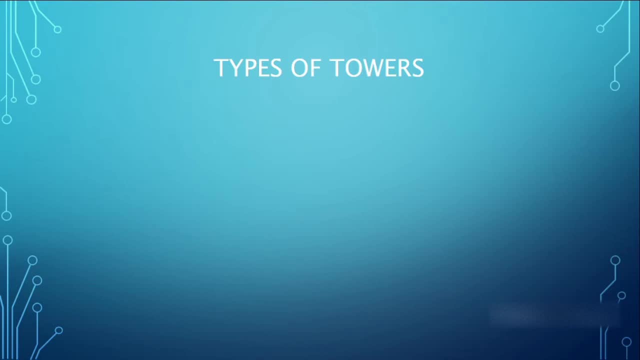 There are different types of towers depending upon the voltage of the transmission line, The number of conductors used, the number of circuits of the transmission line and the physical location of the tower. The main types of towers are suspension tower, tension or detergent tower, and transposition tower. 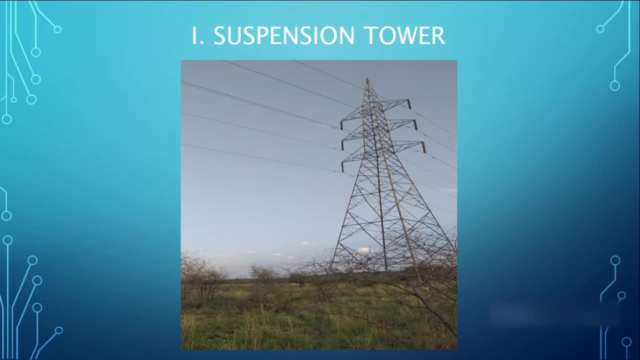 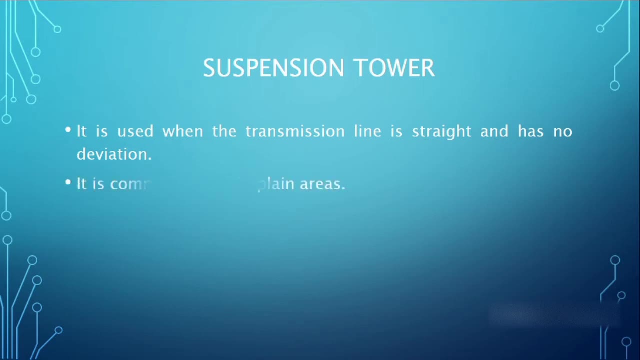 Suspension tower is the type of transmission line tower which is most commonly used. Suspension tower is used when the transmission line is straight and has no deviation. It is most commonly used in plane area. The conductor is hanging from the tower through disc insulators and there are no jumpers involved. 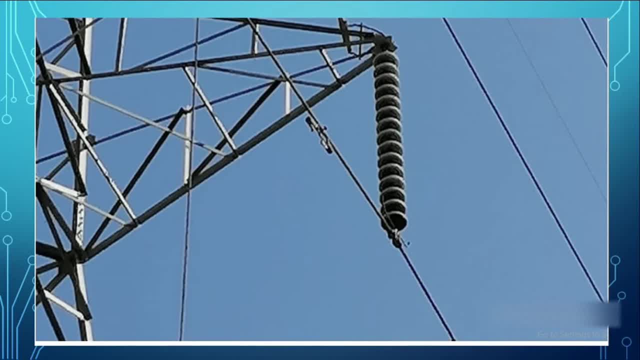 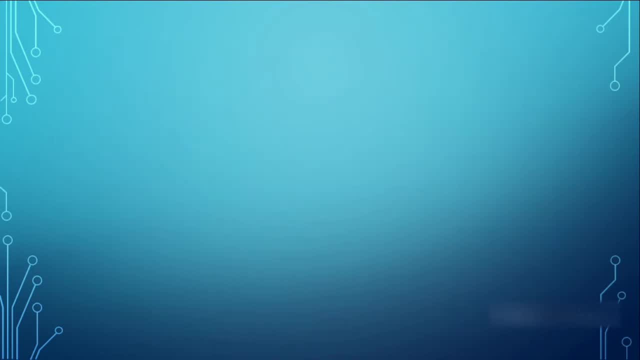 Let's have a closer look of a conductor hanging from a suspension tower. That's how a 500 kW suspension tower looks like. Now we come across the tension or detergent tower. Tension towers are used when there is deviation required in the transmission line and the transmission line is not on straight. 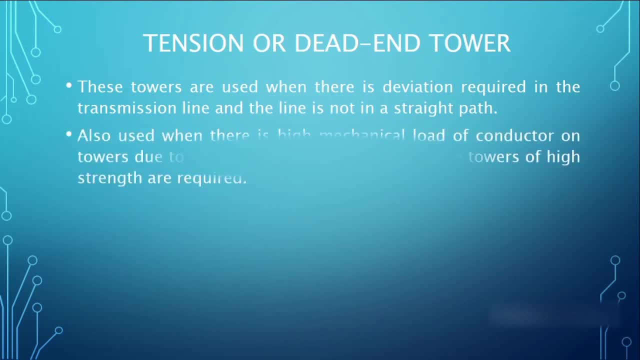 path. Tension towers are also used when there is high mechanical load on towers due to tough terrain, For example hilly areas, And where more strong towers are needed. In tension towers, conductors are not hanging from the towers like normal suspension towers. 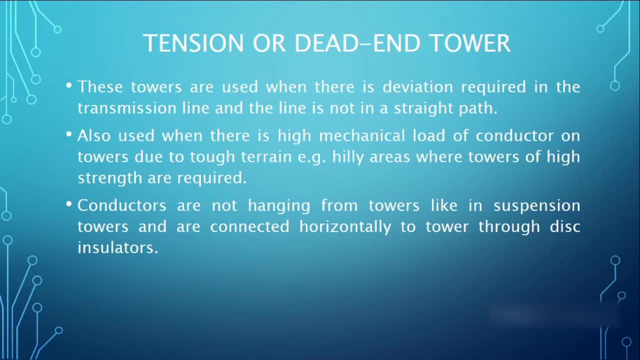 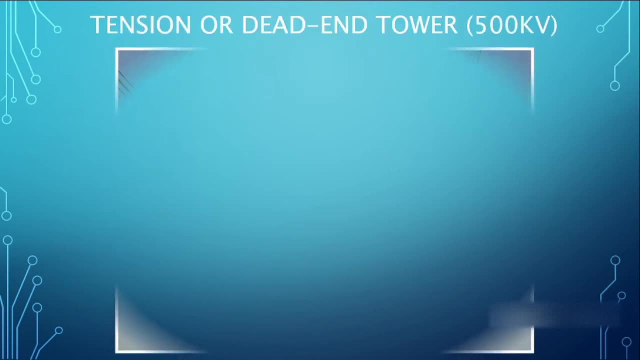 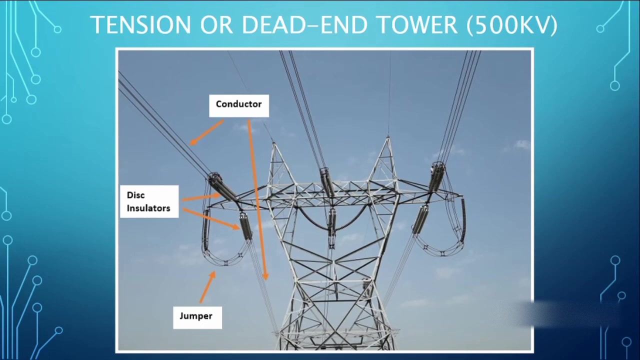 but are horizontally connected to tower through disc insulators. Jumpers are used to connect the conductors on both sides of the tower. That's how a 500 kW detergent tower looks like. We can see the conductor, disc insulators and jumpers in the tension tower. 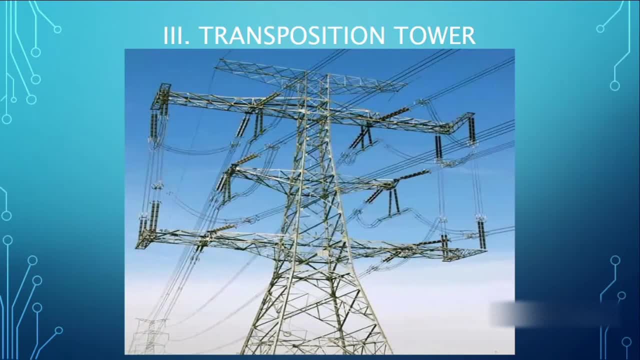 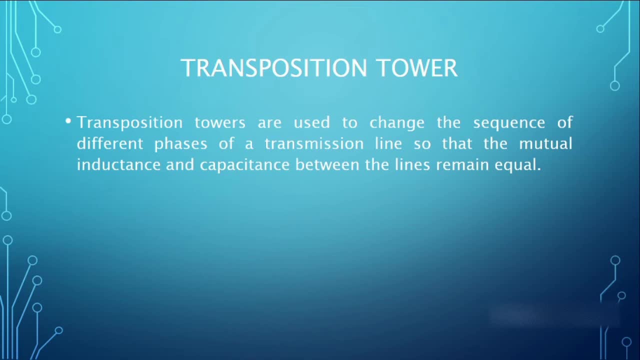 Next we explain the transposition towers. Transposition towers are used to change the sequence of different phases of a circuit so that the mutual inductance and capacitance between the lines remain equal. Transposition is normally done on very long transmission lines and normally done at two. 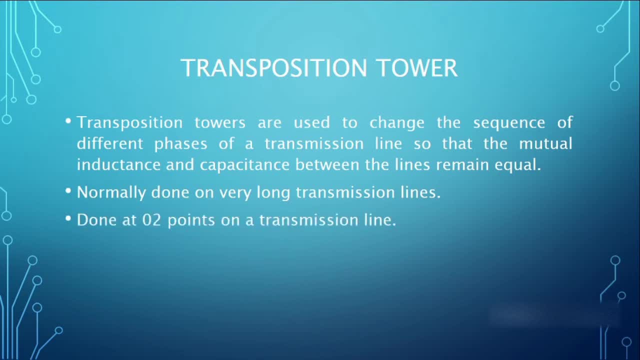 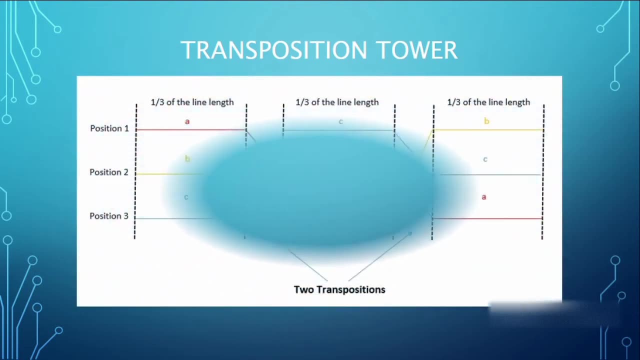 points on a transmission line. The transposition balances the capacitance of the transmission line, which results in balancing of the voltage. This graph explains that how transposition works. We can see that transposition is done at two points in this graph. The red, yellow and blue phase changes their positions at. 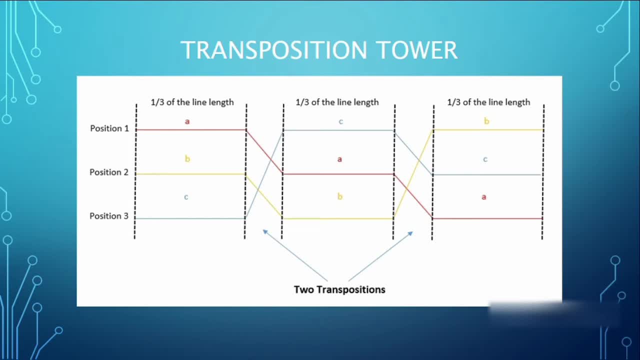 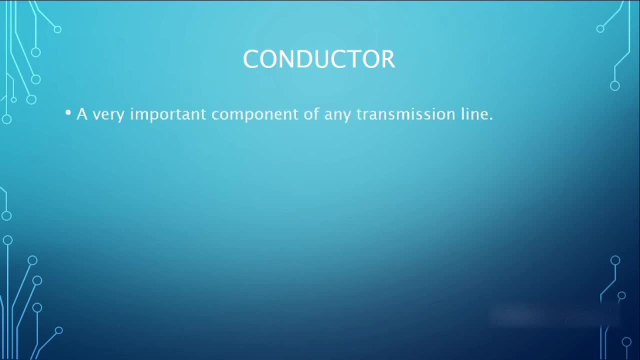 transposition points which help in balancing the line. capacitance Conductor is another very important component of any transmission line and extensive care is required for the selection of suitable conductor for electric power transmission. There are different types of conductors based on the voltage level of the pot being transmitted. 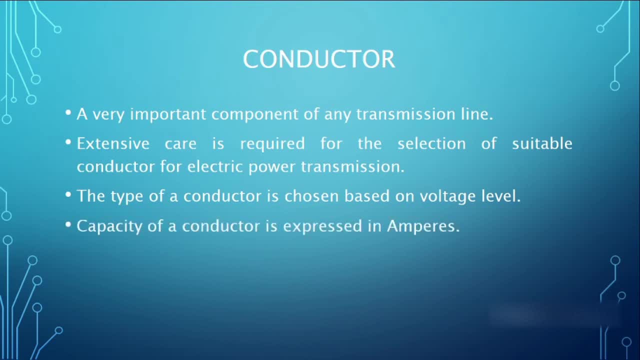 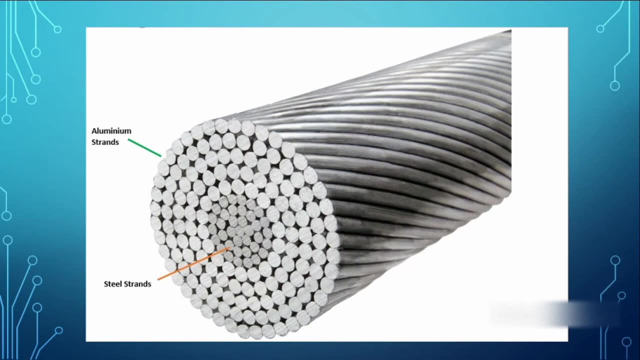 Capacity of a conductor is normally expressed in amperes. A conductor is composed of a number of strands. This is an ACSR conductor. We can see the steel strands in the middle surrounded by the aluminum strands. Normally for high voltage transmission lines ACSR and triple. 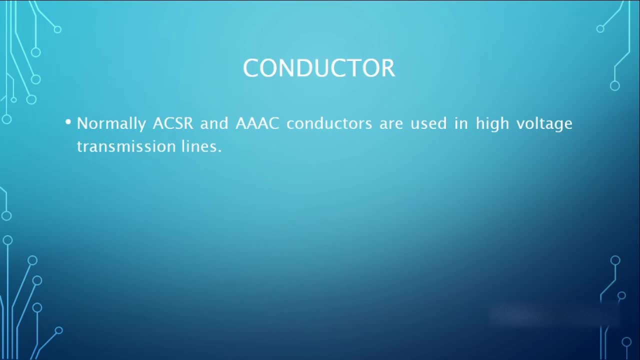 AC conductors are used. ACSR stands for aluminum conductor- steel reinforced, whereas triple AC stands for all aluminum- alloy conductor. The conductors vary according to the number of strands of aluminum and steel and the diameter of the strands. Aluminum is a very good conductor of electricity, whereas steel is good for providing mechanical 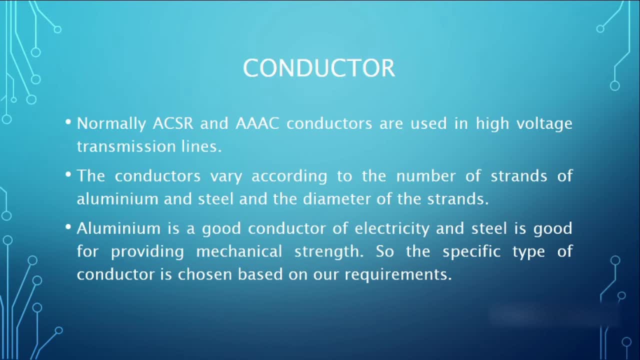 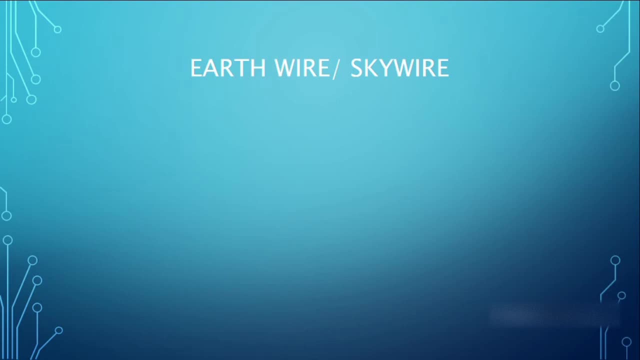 strength. So the specific type of conductor is chosen based on all requirements: Earth wire or sky wire. Earth wire is used to provide protection against lighting or thunder strikes. These days, OPGW wire is mostly used instead of normal sky wire. The benefit: 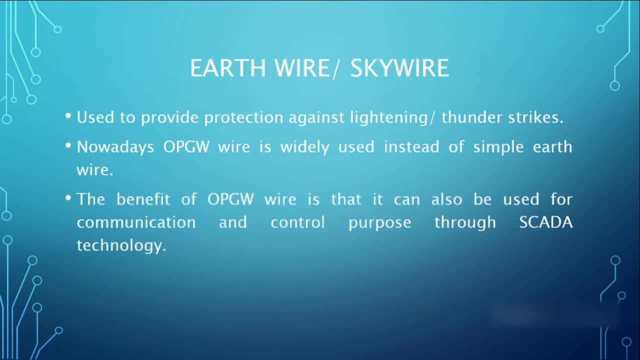 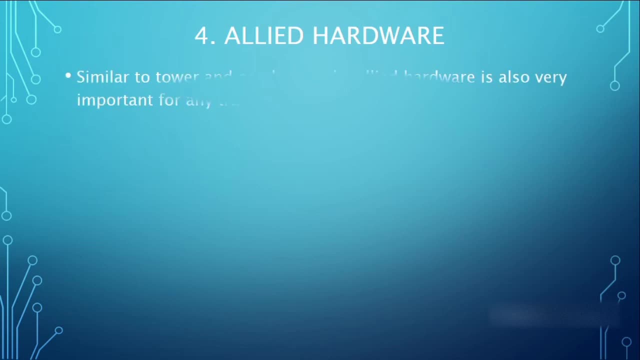 of OPGW wire is that it can also be used for communication and control through SCADA technology. Allied hardware Similar to tower and conductors. the allied hardware is also very important for any transmission line. Without the allied hardware, any transmission line is incomplete. Some of the main allied 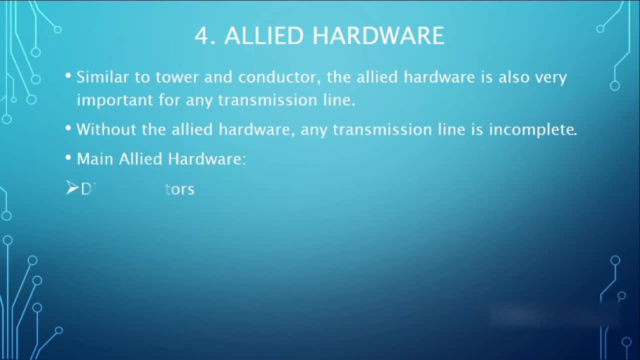 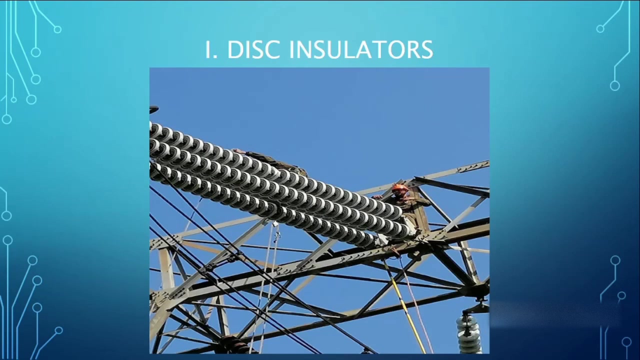 hardware are given as below: Number 1. Disk insulators. Number 2. Spacers. Number 3. Damper weights. Number 4. Dead end bodies. Number 5. Arcing Ons Disk insulators. Disk insulators are used to provide insulation.